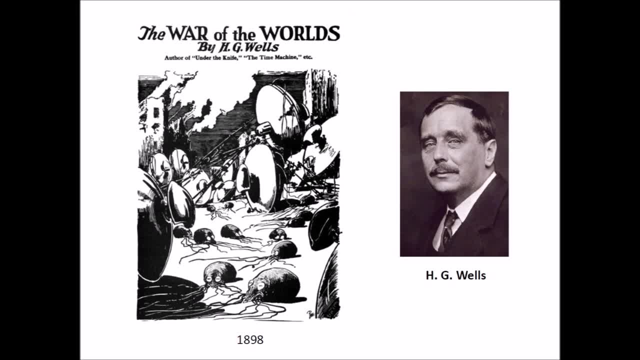 novels of a conflict between mankind and an extraterrestrial race. The book describes the invasion of southern England by Martians with advanced technology. A live broadcast of a drama based on this book on October 30, 1938 caused panic among the listeners in the United States. 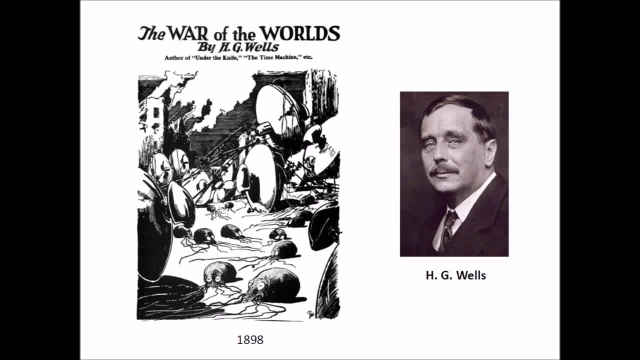 because they thought that the Earth was really being invaded by Martians. It is reported that at 8.50 pm a huge flaming object believed to be a meteor was being destroyed in the Earth. meteorite fell on a farm in the neighborhood of Grover's Mill, New Jersey, 22 miles from. 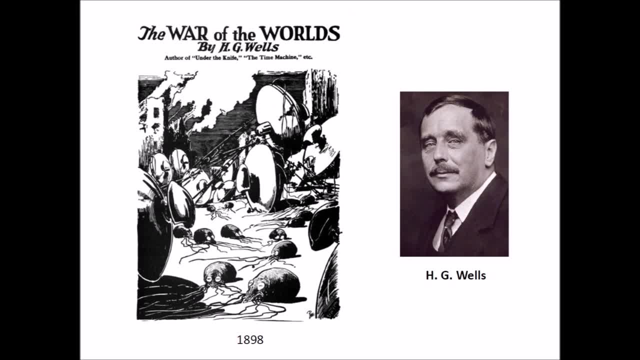 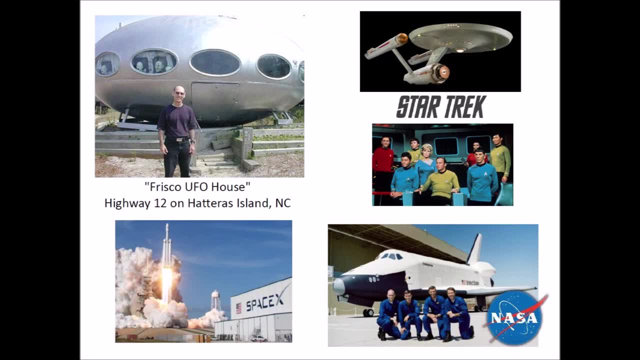 Franklin. There is a link to this radio program in the description below. Currently, the space industry is making great strides with communication satellites, weather satellites and space stations. Space exploration is shifting from being sponsored by government agencies to private businesses like SpaceX. Science fiction has provided inspiration for the space industry. 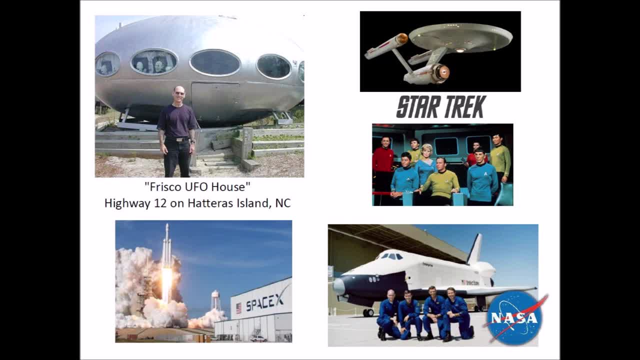 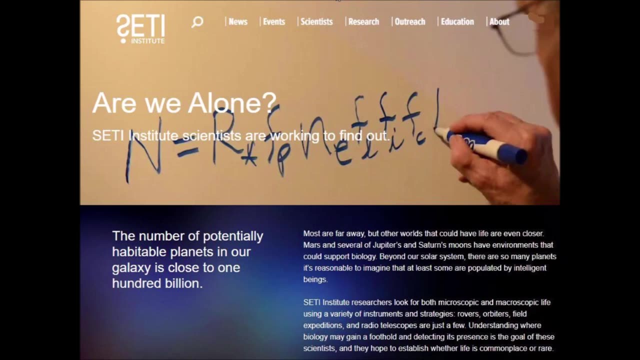 The Space Shuttle Enterprise was named after the Starship Enterprise from the Star Trek television series. The idea that there are intelligent extraterrestrial species is more popular today than ever before. The SETI Institute is a research organization incorporated in 1984 whose mission is to explore. 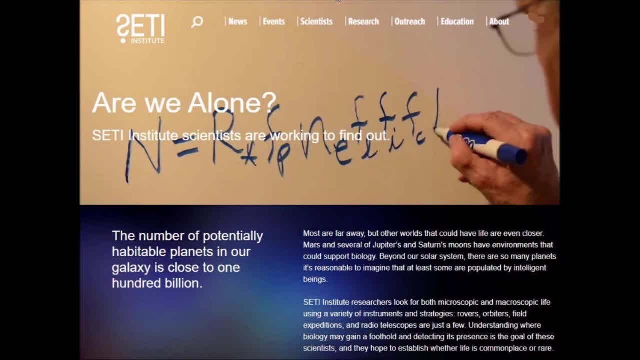 understand and explain the origin and nature of life. The SETI Institute began as a NASA program. Over the years, other research disciplines have been added by their relevance to the search and understanding of life beyond Earth. Today, the Institute has approximately 100 scientists. 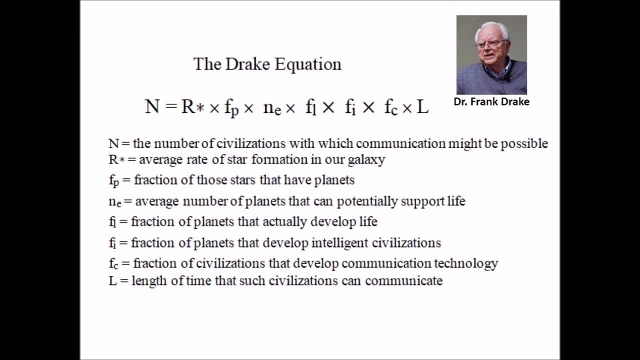 In 1961, American astronomer Frank Drake, who was the founder of the SETI Institute, proposed a probabilistic equation to stimulate scientific dialogue about the search for extraterrestrial intelligence. The equation estimates N, which is the number of civilizations in the Milky Way galaxy whose 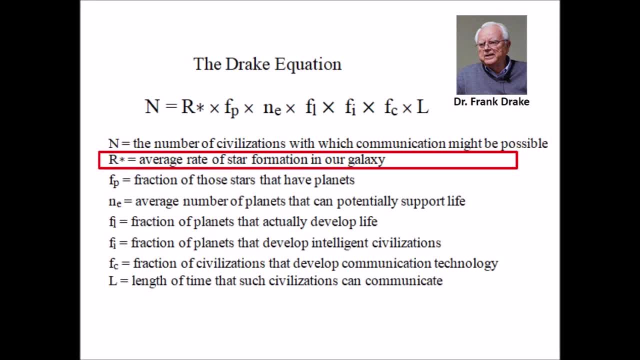 electromagnetic emissions are detectable. R star is the rate of formation of stars suitable for the development of intelligent space. The SETI Institute is a research organization incorporated in 1984, whose mission is to explore, understand and explain the origin and nature of life beyond Earth. Aquí tenemos una suma muy interessante del carbohidrógico y la esperanzadora de la investigación. Fp is the fraction of stars that help planets. Ne is the number of planets per solar system that can potentially support life. Fl is the fraction of suitable planets that actually develop life. 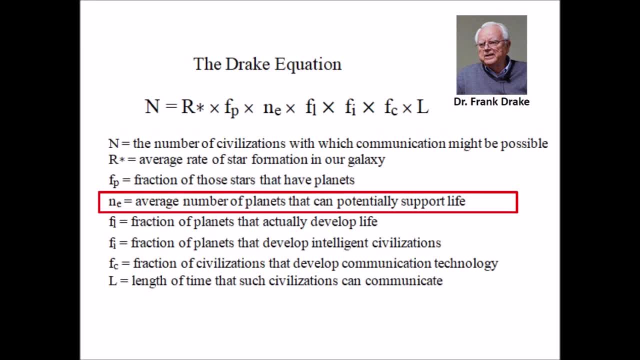 Fi is the fraction of planets that develop intelligent civilizations. Fc is the fraction of intelligent civilizations that develop electromagnetic communication technology. L is the average length of time during which such civilizations can develop intelligence systems. such civilizations can communicate. Unfortunately, the values for the factors are very difficult. 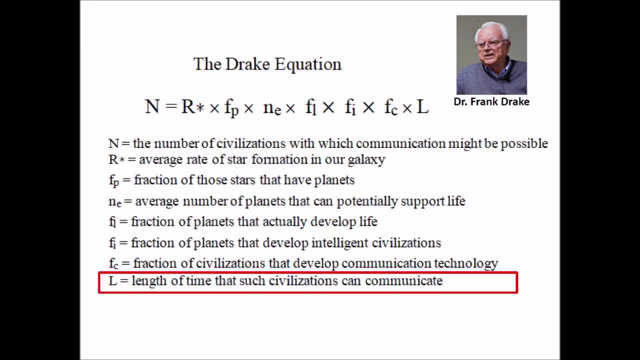 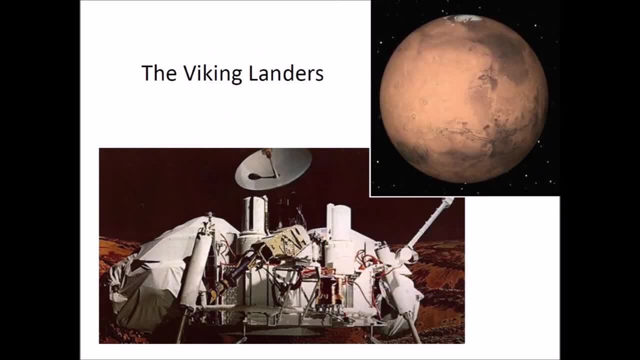 to estimate and the uncertainties are so large that the equation cannot be used to draw firm conclusions. In 1976, NASA sent the Viking 1 and Viking 2 space probes to Mars with four types of biological experiments. Of these experiments, the labeled release experiment returned positive results on both landers. however, the controlled 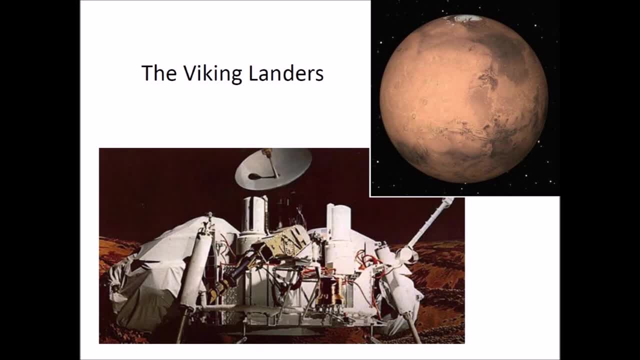 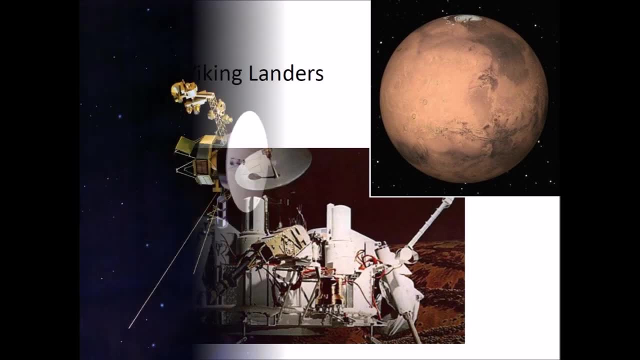 tests could not confirm the results. We may have already found bacterial life in Mars, but we cannot say for sure. Future missions will be needed to verify this. In 1972, the United States launched Pioneer 10.. This was the first mission to the planet. 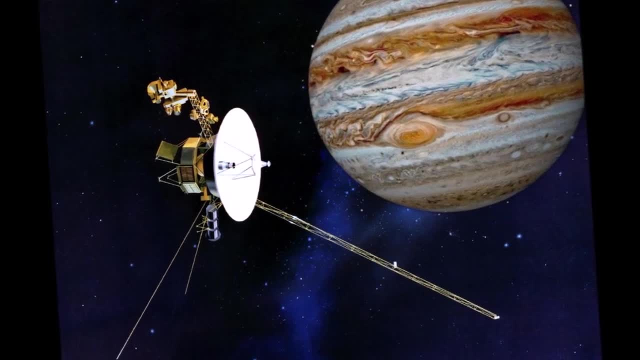 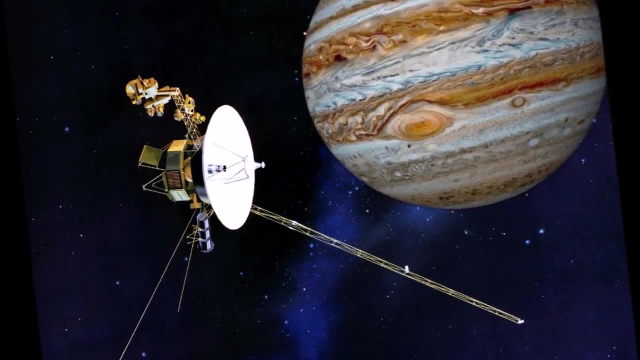 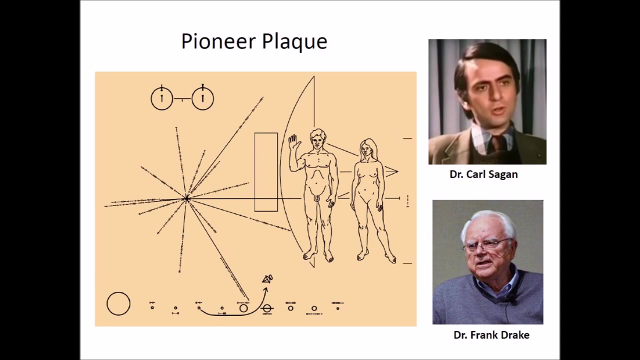 Jupiter. After getting a gravitational boost from Jupiter, Pioneer 10 became the first artificial object to achieve the escape velocity needed to leave the solar system. The Pioneer spacecraft carried a plaque designed by Carl Sagan and Frank Drake. It depicts a nude man and a woman in front of the parabolic. 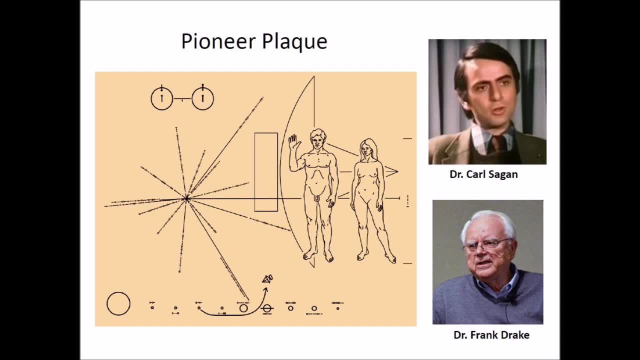 antenna of the space probe, and it includes the planets of our solar system. This was the first physical message sent into space. The plaque was designed to be understandable by extraterrestrials who may encounter it. In an interview with the BBC, Carl Sagan said: 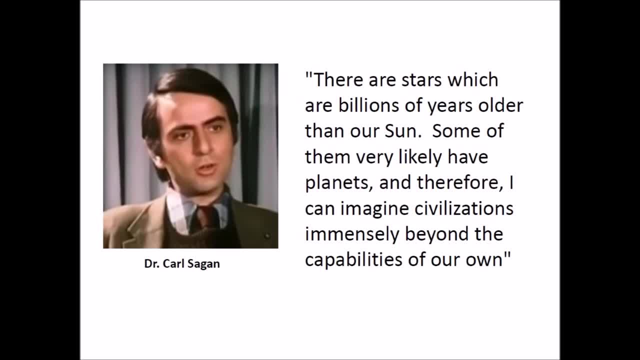 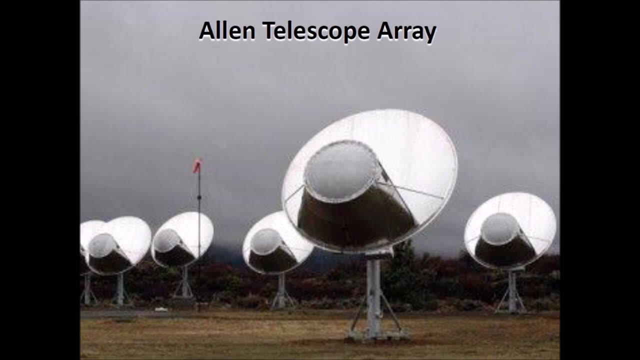 There are stars which are billions of years older than our sun. Some of them very likely have planets and therefore I can imagine civilizations immensely beyond the capabilities of our own. The Allen Telescope Array is a radio telescope array dedicated to astronomical observations and a simultaneous search for extraterrestrial intelligence. The array is situated at the 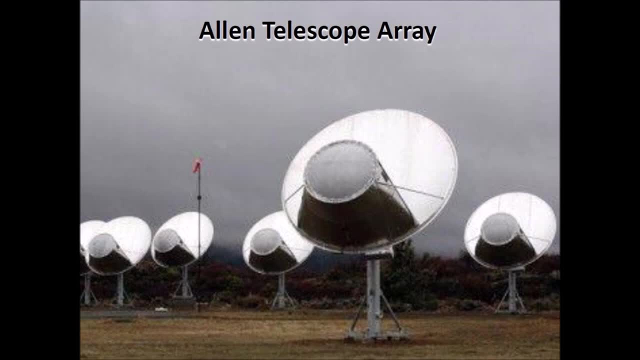 Hatt Creek Radio Observatory, 290 miles northeast of San Francisco, California. The telescope array is named after Paul Allen, a co-founder of Microsoft, who has contributed more than $30 million to the project. In the Star Trek television series, they use a. 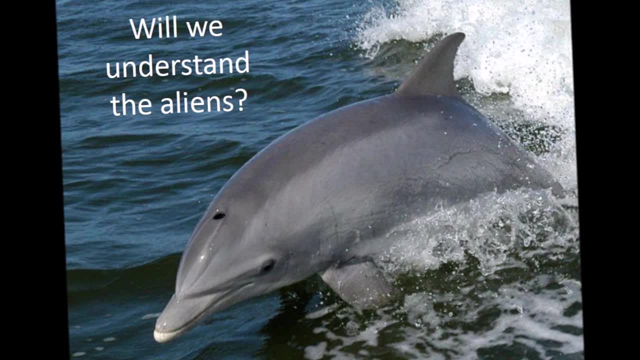 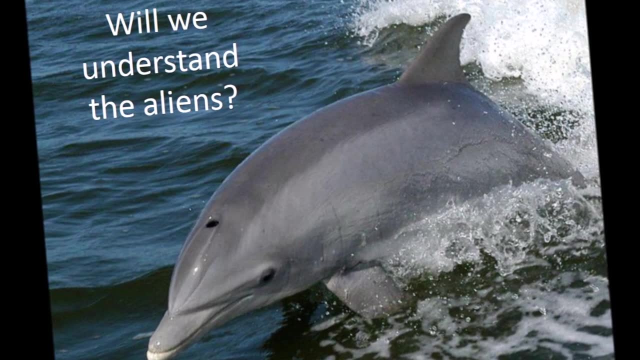 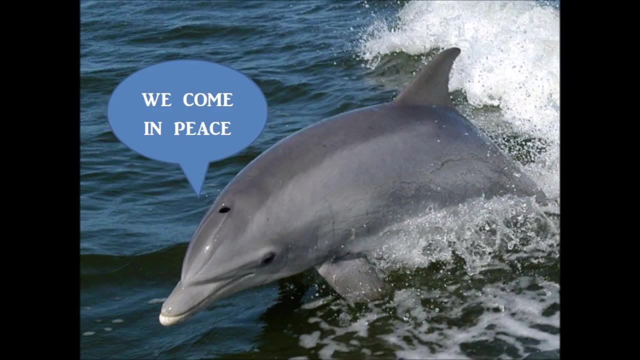 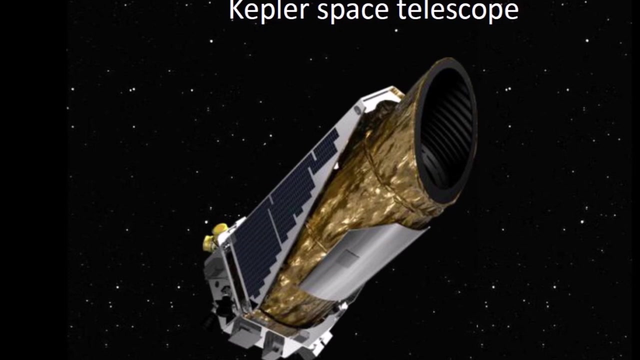 universal translator to talk to the aliens in English. Thus far, we cannot even understand dolphins, who are intelligent and seem to call each other by name. They use whistles and clicks to coordinate their activities, for hunting and to defend themselves from predators. The Kepler Space Telescope was launched on March 7, 2009 by NASA into an Earth-trailing. 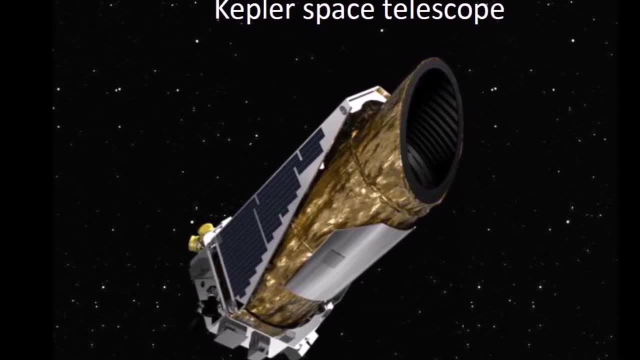 heliocentric orbit. Its mission was to discover Earth-sized planets orbiting other stars. The telescope was designed to detect and detect the Earth-sized planets orbiting other stars. The Kepler Space Telescope was launched on March 7, 2009 by NASA into an Earth-trailing. 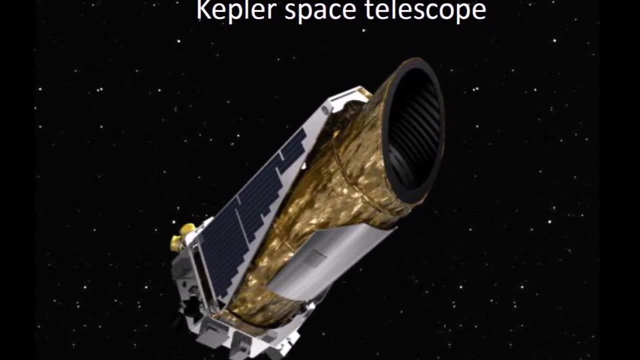 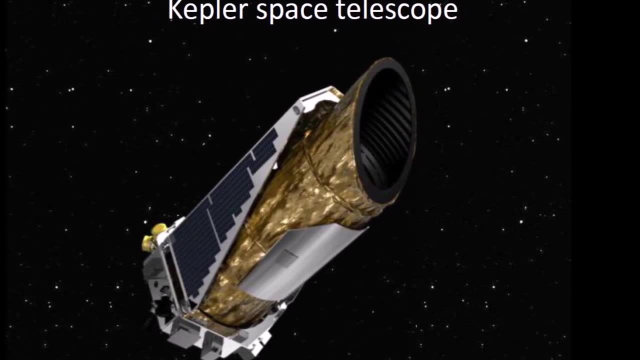 heliocentric orbit. Its mission was to discover Earth-sized planets orbiting other stars. The Kepler space telescope was allowed to get rid of aliens. now we will see why. Kepler's sole scientific instrument was a photometer that continually monitored the brightness of approximately 530,506 stars and detected 2,662 planets during its nine-year. 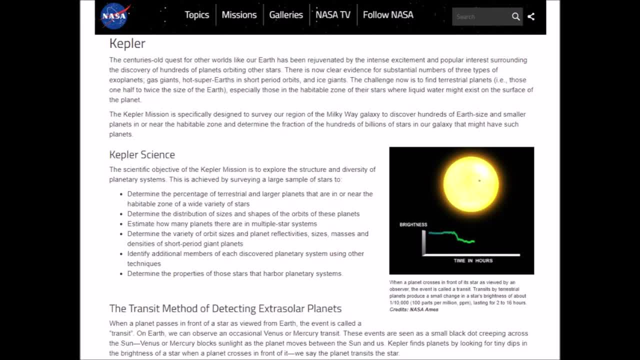 lifetime. The Kepler telescope found planets by looking for the slight dimming of a star caused by the transits of a planet in front of the star. The cyclical patterns of dimming can be used to determine the orbital period of the planet. Mysterious and allocated SQL že libert Марк. 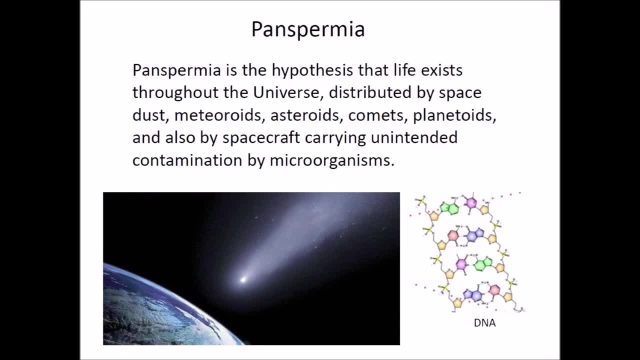 Syfield Computer Education Data Analysis. Manôme Beatles, Ancient、 Hessian Houston Coulut Lanuiâne from utter mystery です and originalнения takat yeahwha bre itu that life exists throughout the universe, distributed by space, dust, meteoroids. 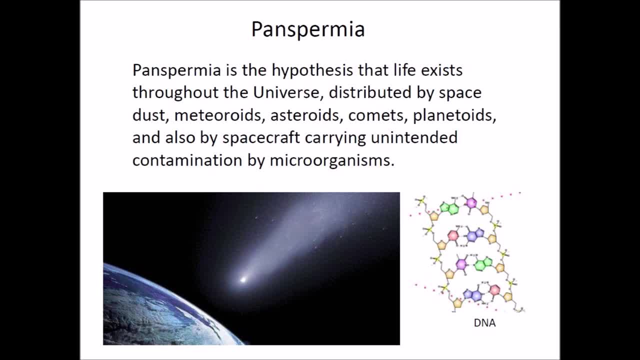 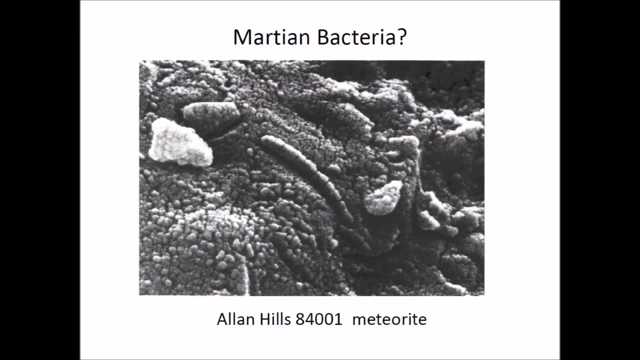 asteroids, comets, planetoids and also by spacecraft carrying unintended contamination by microorganisms. An expedition of meteorite hunters found a meteorite in the Allan Hills of Antarctica on December 27, 1984.. Its chemical composition indicates that the meteorite 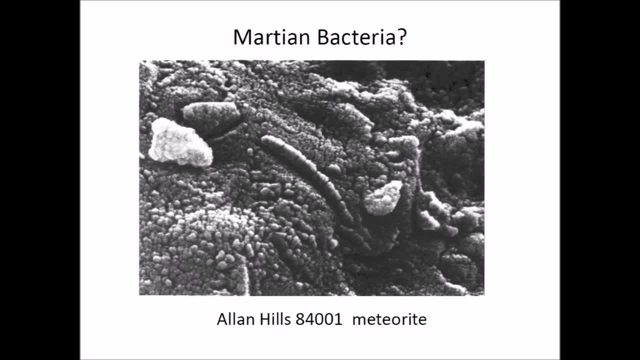 originated in Mars. It is thought that a piece of rock was blasted away from the surface of Mars by the impact of another meteor about 17 million years ago, and it fell on Earth roughly 13,000 years ago. In 1996, a group of scientists claimed to have found evidence for microscopic fossils of 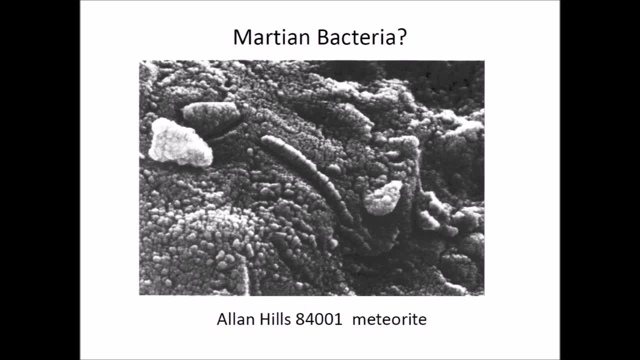 bacteria in the meteorite, suggesting that these organisms also originated in Mars. These findings are very controversial and they have been generally rejected by the mainstream scientists. For now, you will only see scary aliens on TV. But don't worry, the United States is. 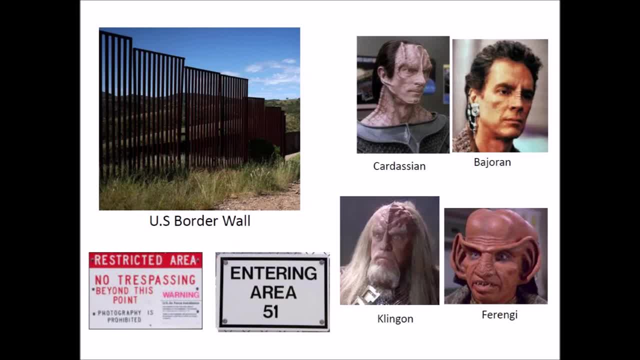 building a new science-fiction project for the future. It will be a project that will bring a border wall that should keep the aliens out, except for Area 51.. Shh, that's supposed to be a secret.